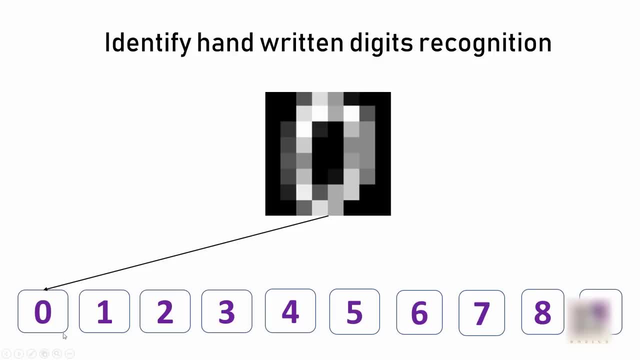 to one of the output categories, which is nothing but digits 0 to 9.. Similarly here for maps to this particular output category. So we will use a training set with a lot of hand digit characters and then we'll build a model using logistic regression. and at the end of the tutorial you 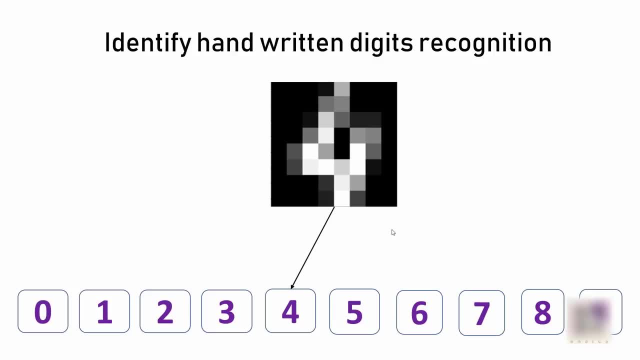 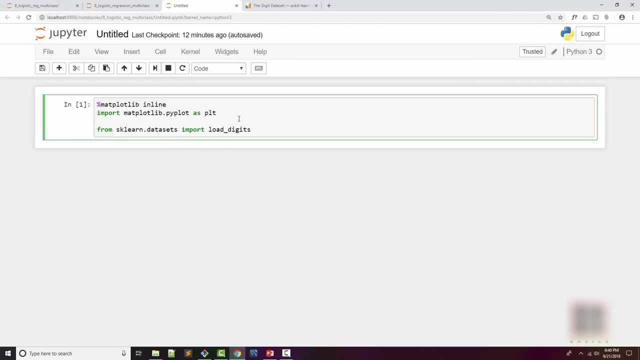 will have an interesting exercise To work on, So let's jump straight into writing the code. As usual, I am going to use my Jupyter notebook as an IDE, and here I have imported matplotlib and also scikit-learn's data set. So sklearndatasets has some predefined ready-made data sets that you can use to learn. 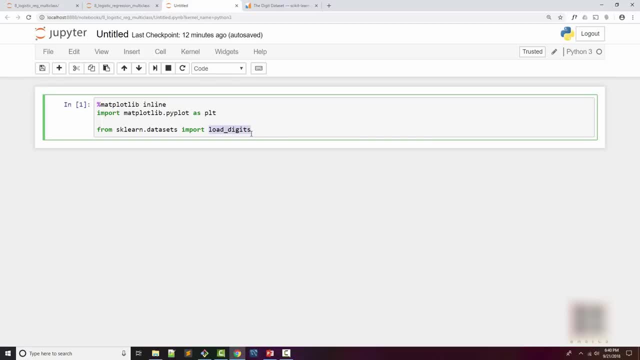 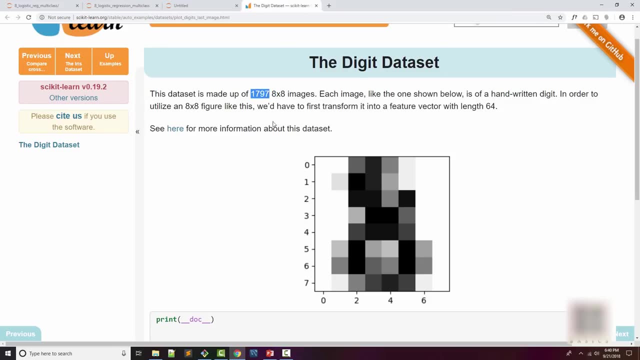 machine learning From this. I am using load digits data set. So if you read the documentation, all it is is 1797 handwritten digits of size 8 by 8.. Okay, so it looks something like this and what we are going to do is, given these digits, we are going to identify that what, what digit? that is All right. 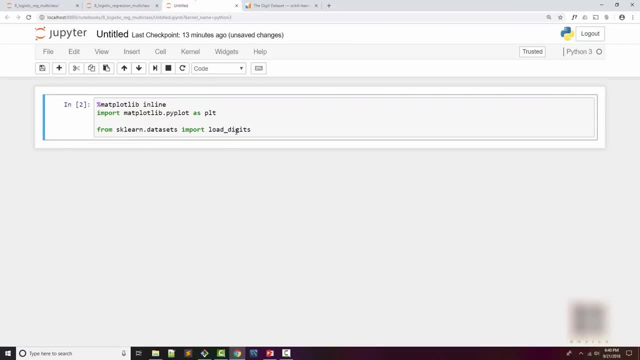 so let me just run it. So this has run fine. I am going to now call load digits method to load my training set, basically, And I want to explore what this training set contains. It contains a couple of things. It has data, which is your real data. 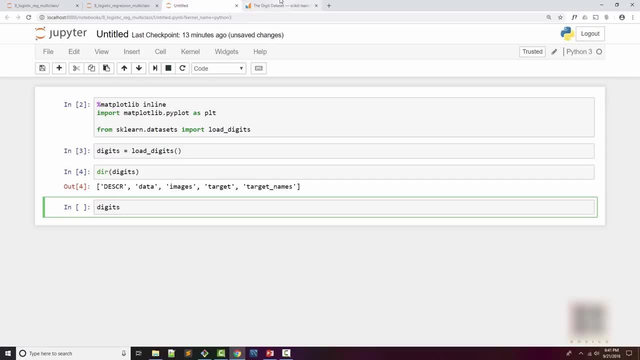 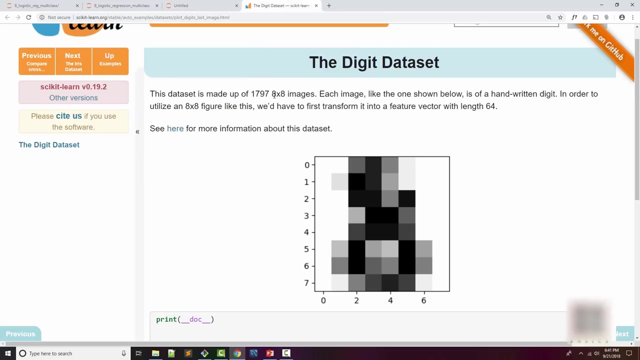 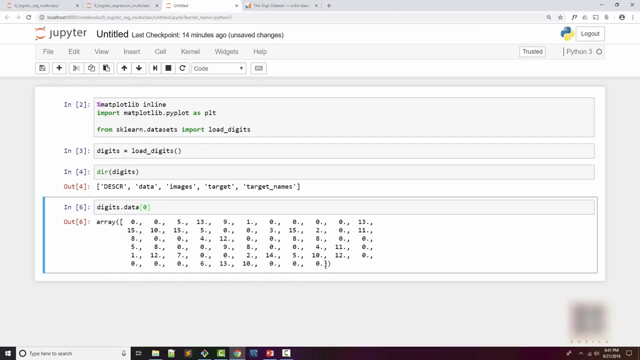 So let's print few elements. So, as it's written in the documentation, there are 1797 sample, So I'm just going to print the first one And it's an array. Okay, As such, it is an 8 by 8 image, But the image is represented as a one dimensional array. So if you count these elements, it will be 64, which is 8 by 8.. 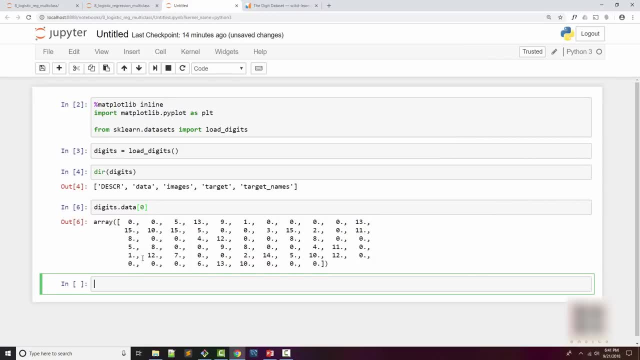 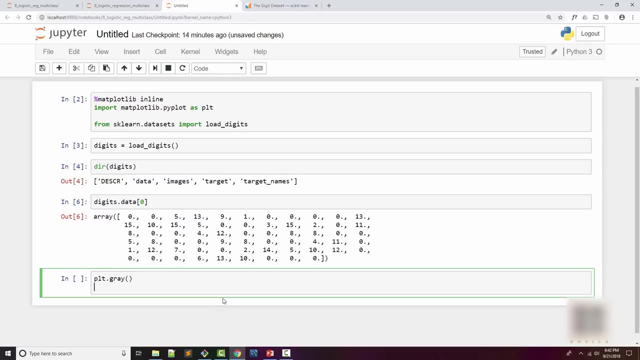 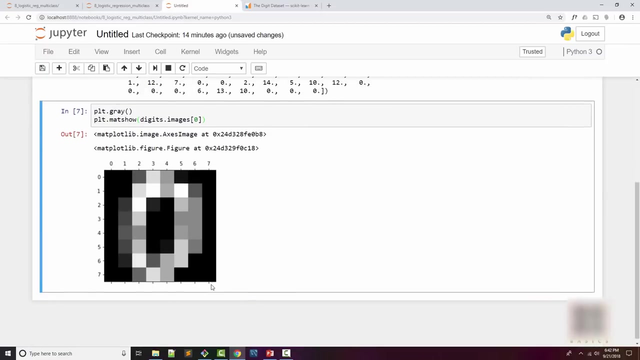 And if you want to see this particular element then you can use matplotlib. So I'm going to do plot pltgray. It is underDEFOL. You can print the corresponding image. so data has the numeric data and image will have the actual images. So you can see that. 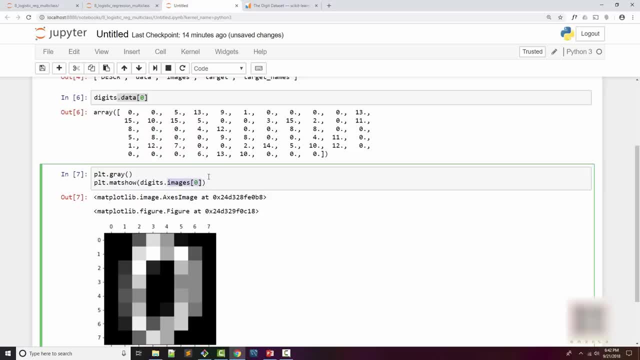 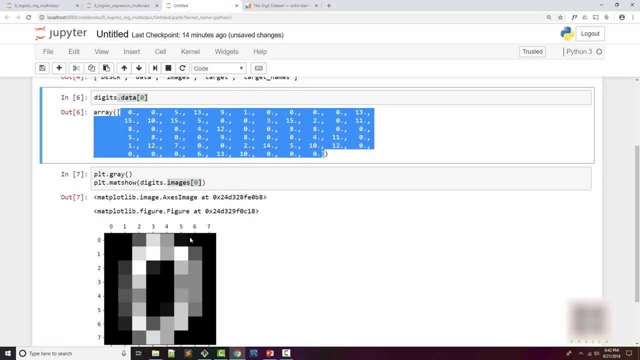 Data 0 and image 0. they kind of relate to each other And the only difference between the two is that you have an American numeric data right here, versus you have an actual image. so if you want to print, let's say first five sample. 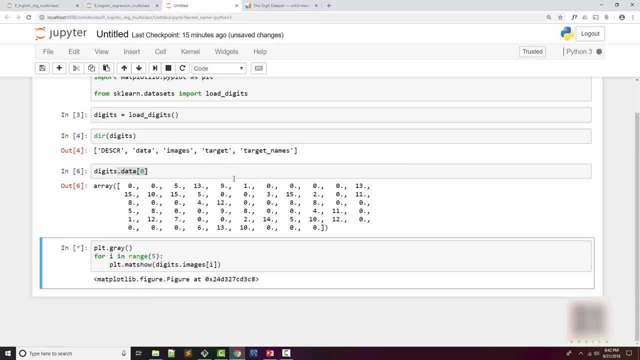 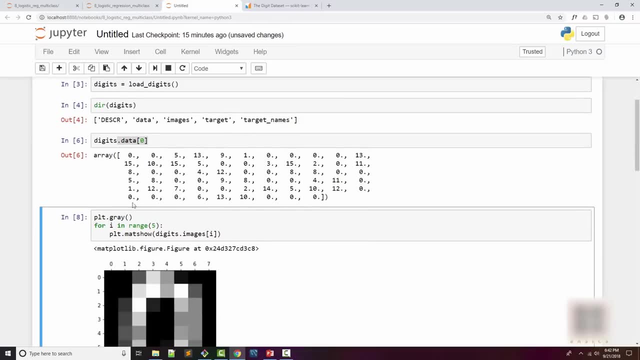 then you can just print it like this and you will see that: see zero, one, two, three, four, okay, and corresponding numbers will be in this data array. so that looks pretty straightforward. now what we are going to do is use this uh to train our model. now, before we do that, let's uh: 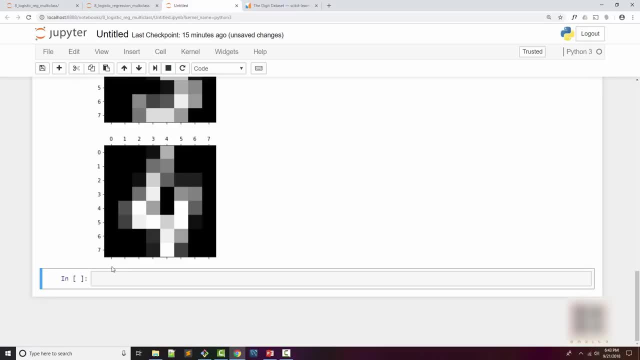 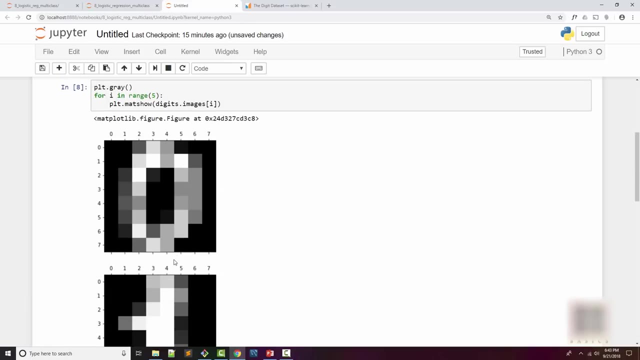 take a look at target and target names. okay, so our target. so if i print digits, dot, target zero, let me print 0 to 5.. so you see, like 0 to 5 is literally in the sequence, the first element is 0, 1, 2, 3 and that's what. 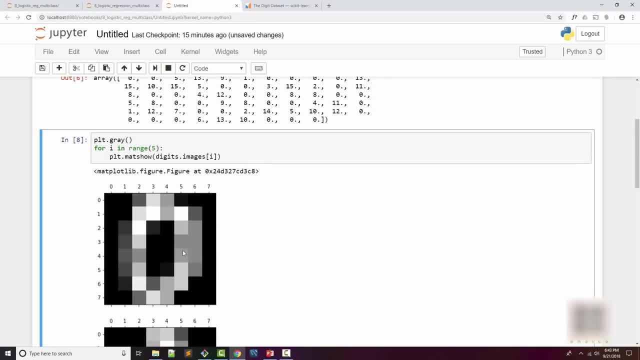 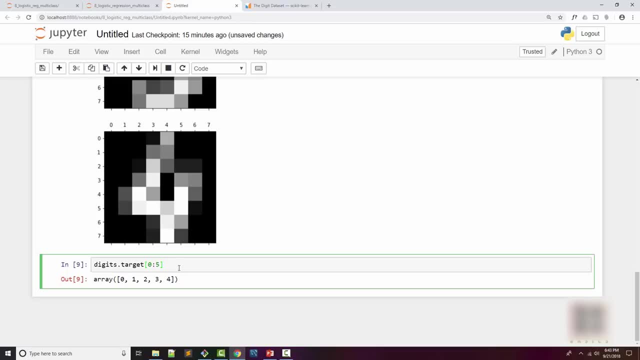 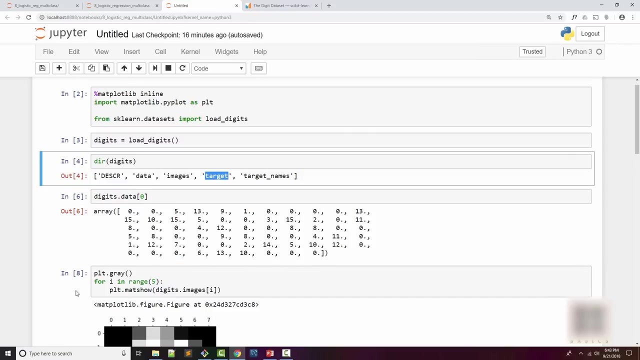 this is printing here. it is saying that this image is zero. the last image, this is four. so this is our complete training set, which has our image as well as the target variable. you know like it says what it is, so we can use our data, data and target to train our model. now, before training our model, 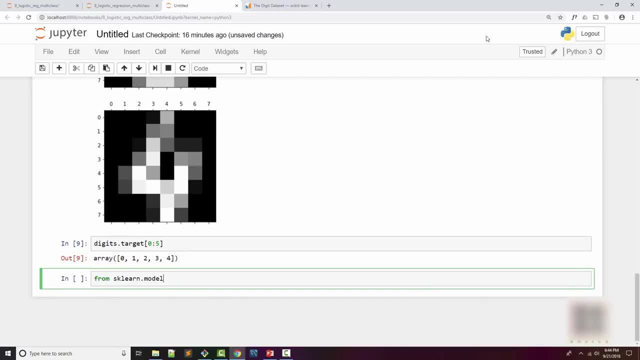 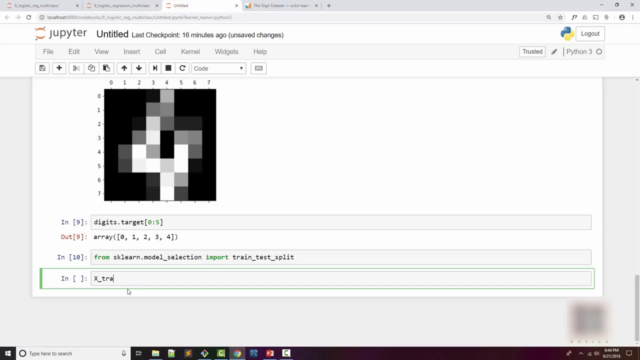 the usual thing that we do is we import from model selection, we import train taste split and we try to divide our data set into a training and taste samples. so the way you do it is you say x train, x taste. i don't exactly remember the order of the argument, so i'm going to what i'm going to do it okay, let me do. 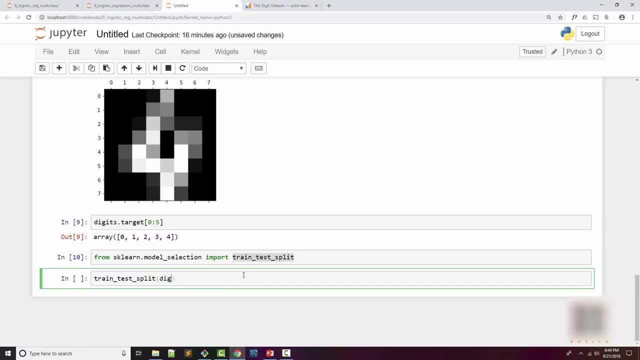 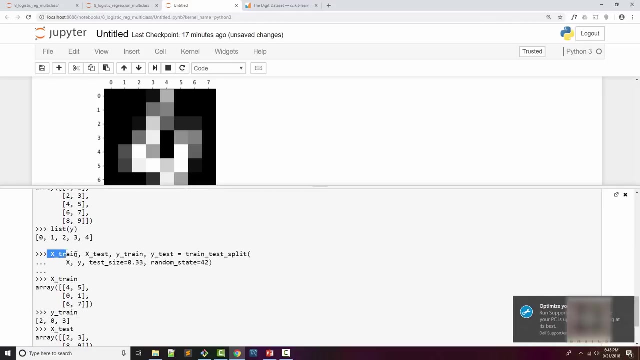 this. so train test split: digits dot data, because that's your data set. then you have digits dot target, because that's your target variable. okay, and if you hit shift tab it will show you all the nice documentation of that api. so here it says: this is the order in which it returns the output. 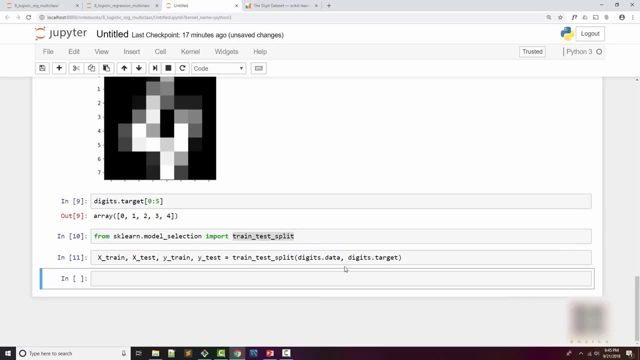 all right. so now, what i just did by executing this command is i had input and output variable from my training set and i divided them into test and train sets. now, the reason that we do this typically is we don't want to, uh, overfit our model. 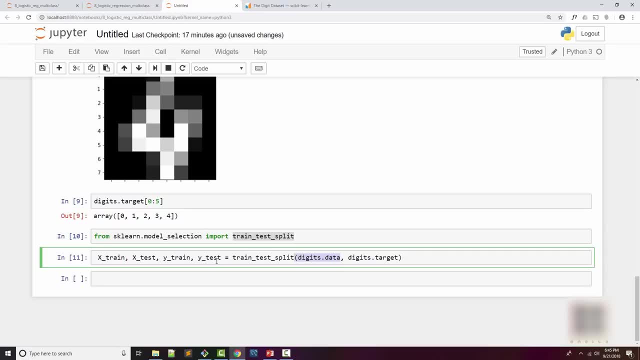 model. we don't want to make our model such that we just bias it against the training data. that's why the data that the model is trained against should be different than the data that the model is tested against. okay, so that's why we split these two. so if you look at, okay, I have to supply the size, so I'm going to. 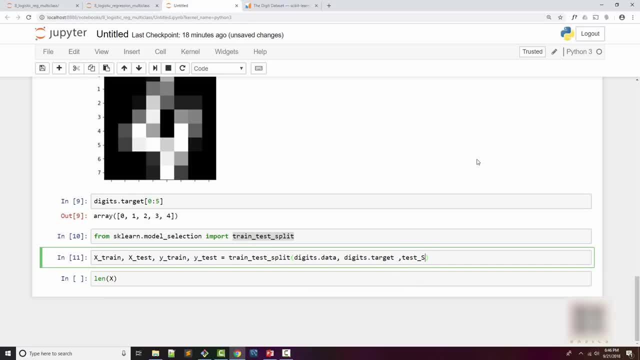 probably supply test size, test size. so I want 20% of my samples to be test size and 80% to be the training. okay, so if I look at length of X train, it is this: and if I look at the length of X days, it is this: 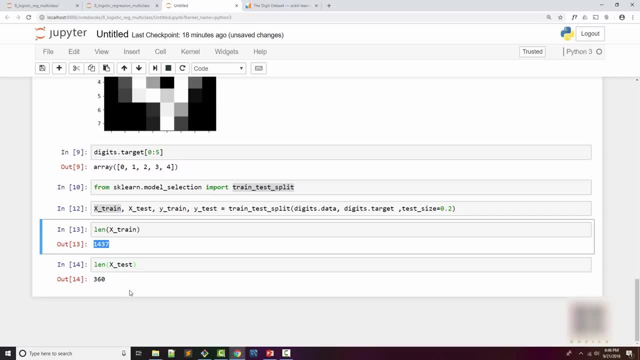 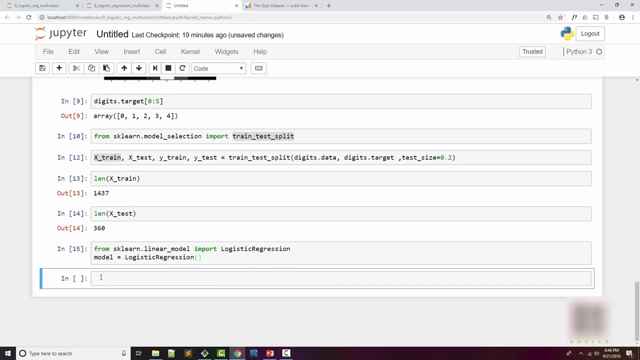 so this is roughly 80% of all available samples. alright, so I have training and test data set split. now I can create my logistic regression model. so from this I want to import logistic però and create a model object so that you can train it later and you all know the way you train it. 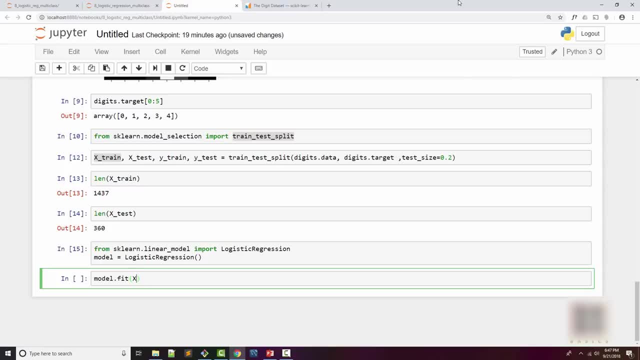 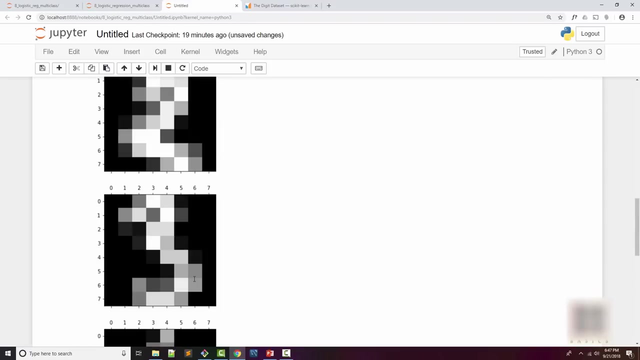 is by calling a fit method and fit method. you will call it against X taste, X train, sorry, and Y train when you run that the model is getting trained using this X train and Y train data set. so again, to repeat, X train has the hand written characters and Y train will have the corresponding. 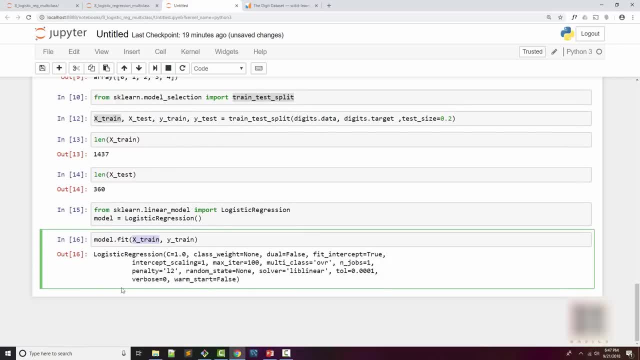 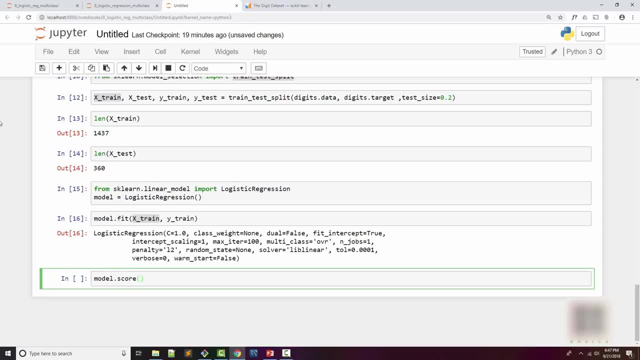 output. it will say: okay for this image, it is for, etc. now, since my model is ready, the first thing I always do is I calculate the score. so the score tells you how accurate is your model and the way you do that is. you have to supply X taste and white is so using the X taste. it will calculate. 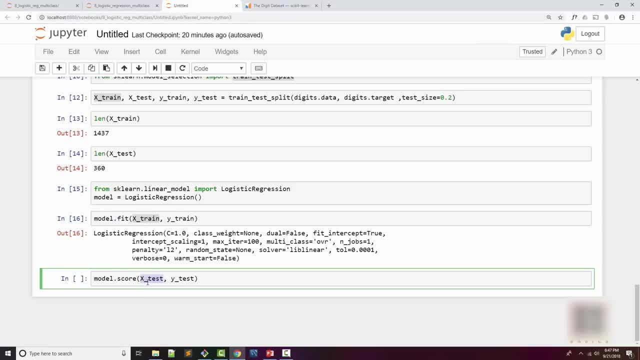 the value of the model and the way you do that is you have to supply X taste and white is. so using the X taste, it will calculate the Y predicted value and it will compare those Y predicted value against the real value, which is Y taste. turns out that my model is doing pretty good. the accuracy is ninety six point. 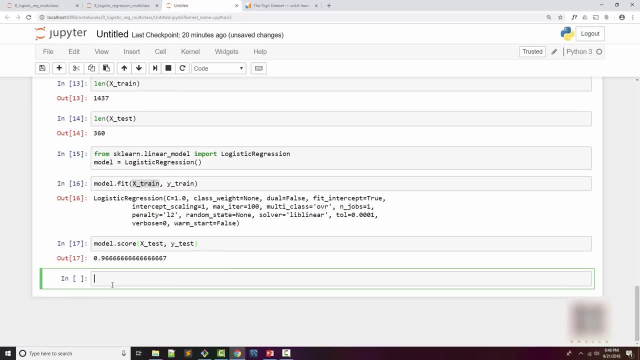 sixty seven percent almost, which is really good. so now I'm going to make my actual prediction, and you know that you have to call predict method for that. now let's see. so before I call this method, what I want to do is I want to pick up a random sample, so I will say PLT, dot, match, show digits, dot. 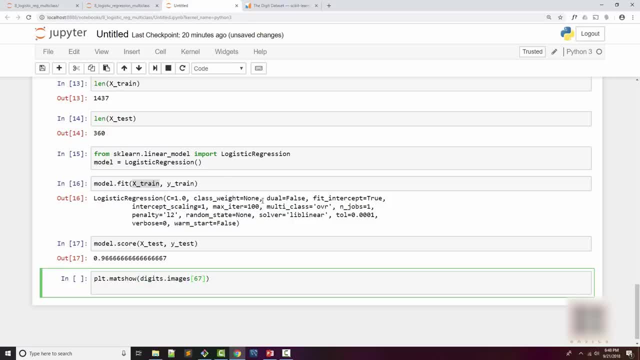 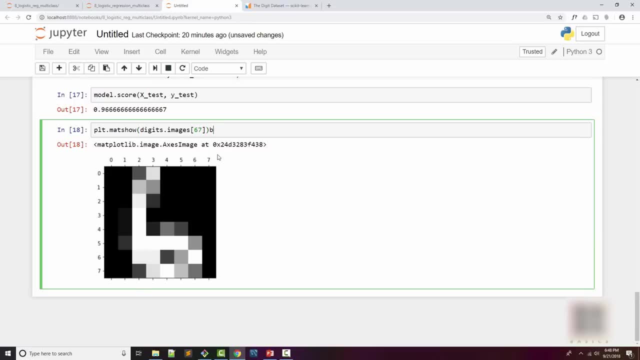 images. let's say I'm just picking up a random sample, okay, hmm, this is pretty hard. even I don't know what this number is actually. let's see. so this number is actually digits: dot target 67. so you have to access the same index in your target. okay, so this is six. okay, so let's see what. 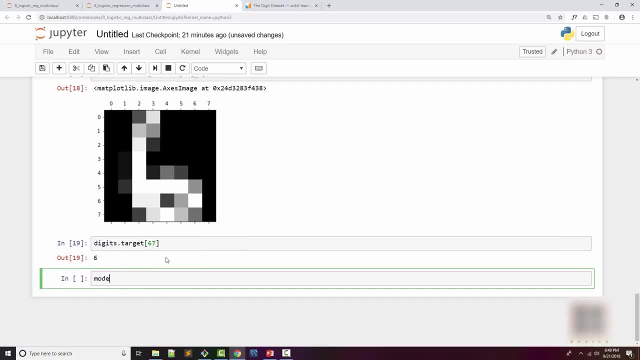 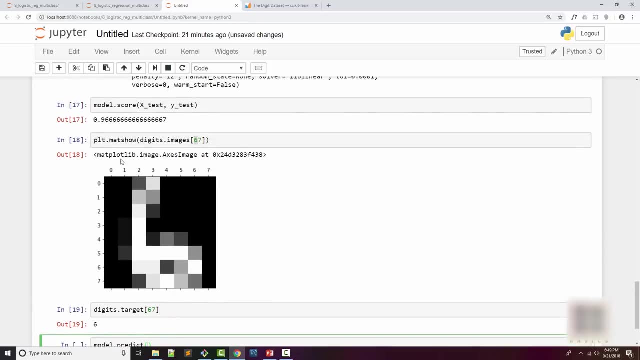 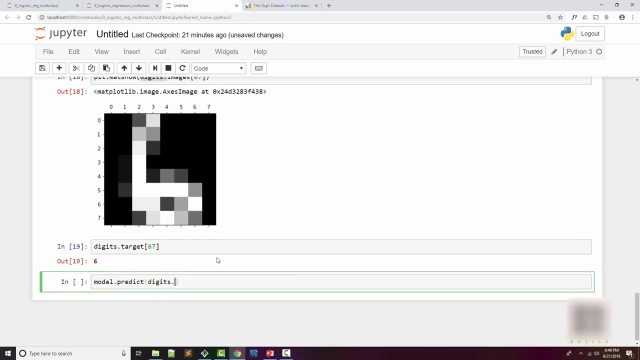 our model will predict for this guy. so I will say: model dot predict, okay, model dot predict what? okay, what do I want to predict? I want to predict. now see, I'm not going to supply images here because image is all is all binary. so I'm not going to supply images here because image is all is all by. 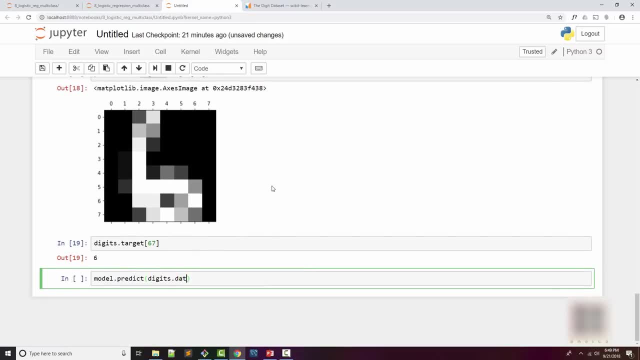 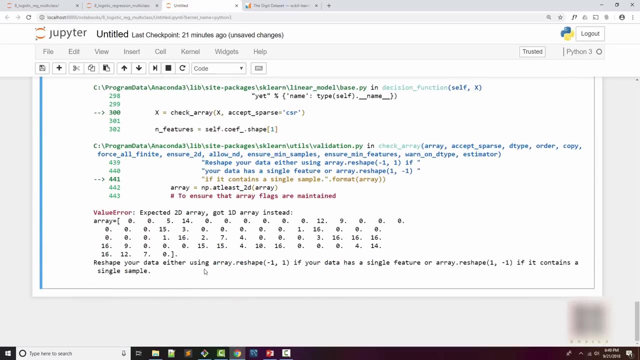 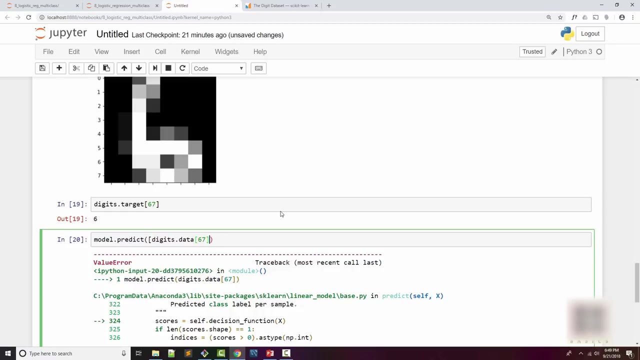 binary data. my model likes numeric data more, so I will use the same index, 67, but I'm using data instead of images. okay, this is the error you get when you are not supplying multi-dimensional array. so I'm just going to supply multi-dimensional array, just for the sake of it, and you can see. 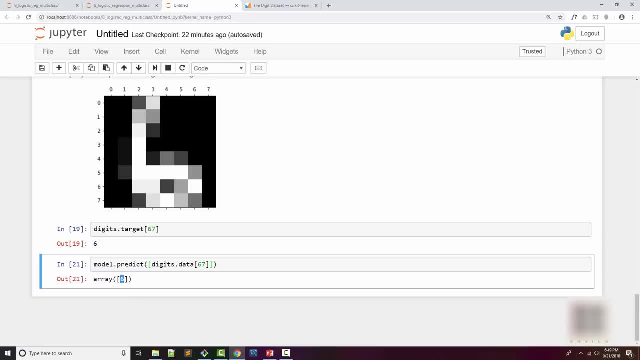 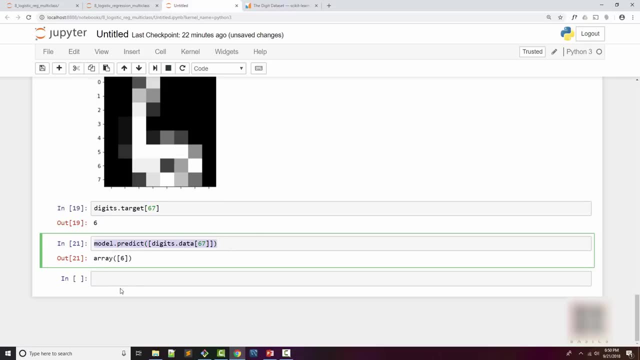 that it is predicting the target variable. all right, okay, let's just okay. let me just create a new cell here and let me predict. okay, what do I want to predict? okay, I want to predict 0 to 5. now, you all know 0 to 5 is. 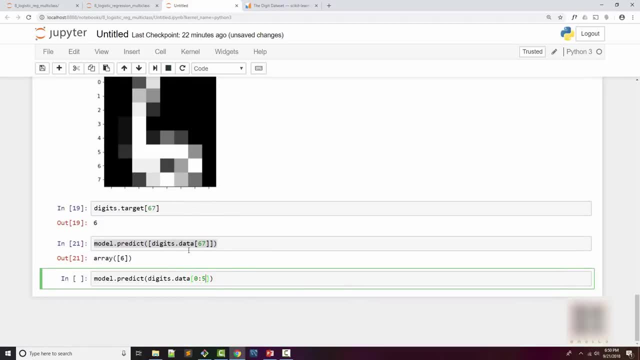 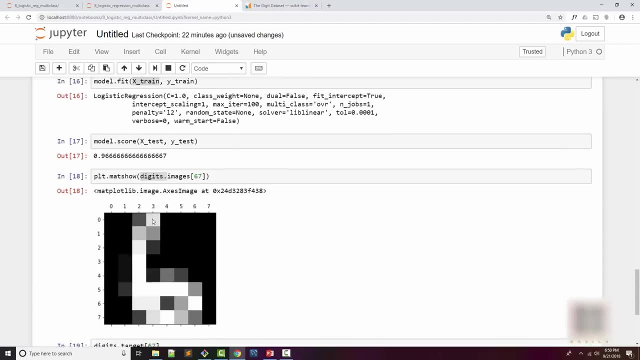 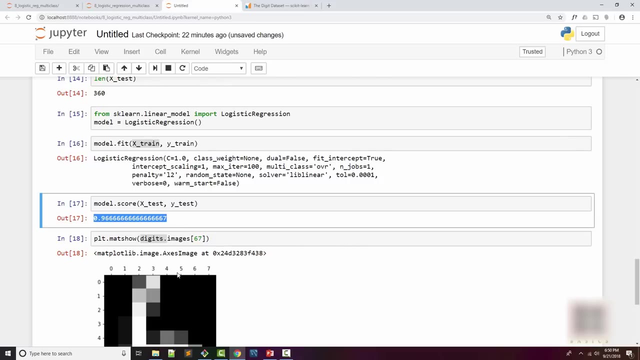 literally 0 to 5, so 0 is 0, 1 is 1 and so on. when executed, see my model is doing pretty good. so well, okay. so my score is 0.96. how do I know where it didn't do? well, okay, because all the Samples I 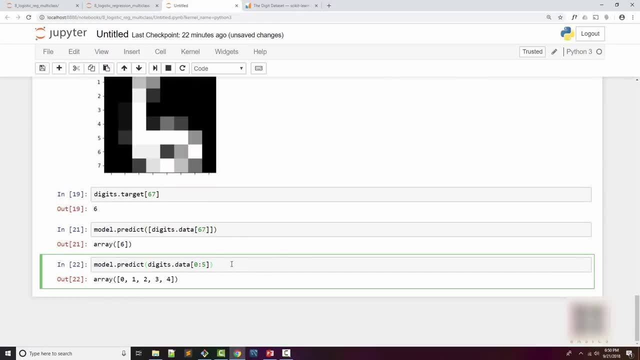 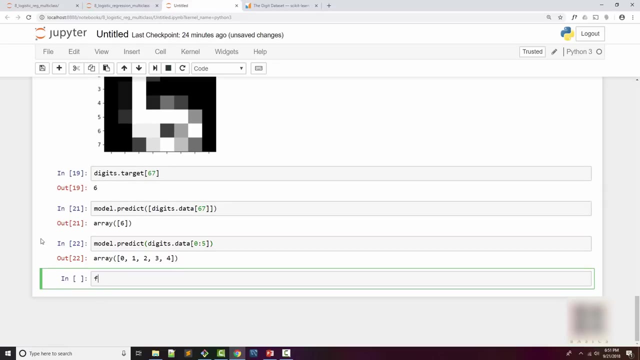 tried. it seems to be doing pretty well. so I want to know where exactly it fail. and you know, I want to get overall feeling of my model's accuracy and one of the ways of doing that is confusion Matrix. so I will show you what confusion Matrix is really now. for that I have to import. 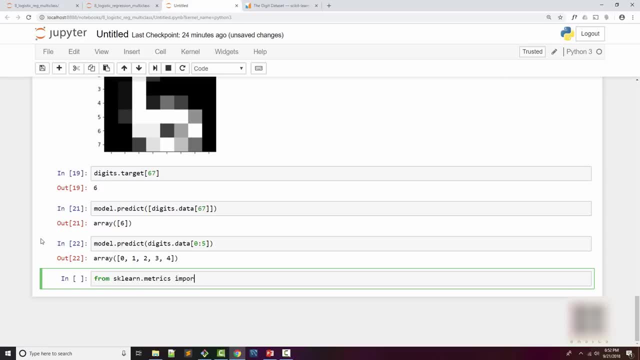 from this matrix. I need to import confusion matrix, okay, and then before I do that I need to get the predicted values. so I will say: predict X taste. when I run that I get all the predicted values for this X taste, okay. and then I create a confusion matrix and in the confusion matrix what you supply is Y. 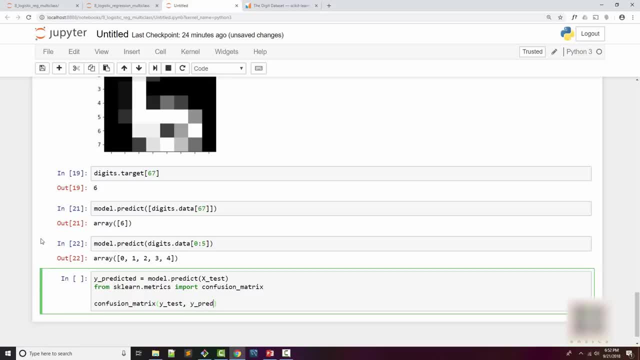 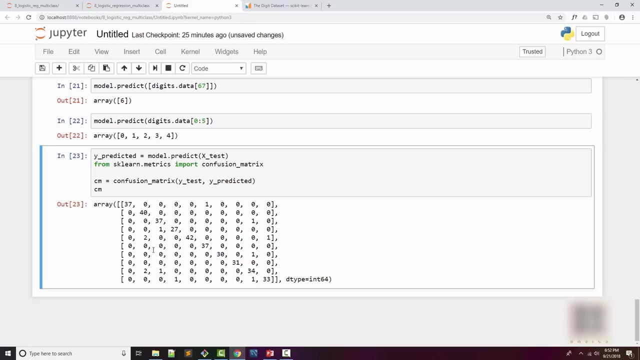 taste, which is the truth, and then Y predicted, which is what your model predicted, and then you get confusion matrix back. when you run that, you get this 2x2 dimensional array and you are wondering what the heck this is. so this is better visualized in matplotlin. 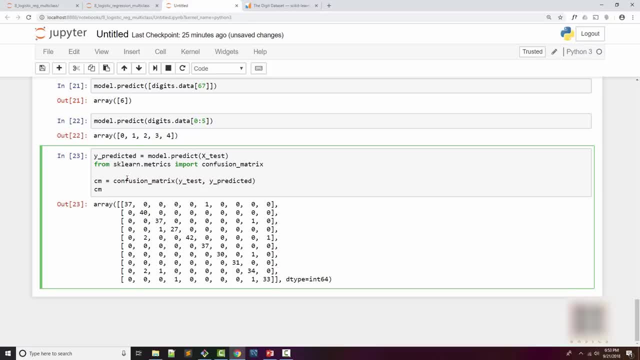 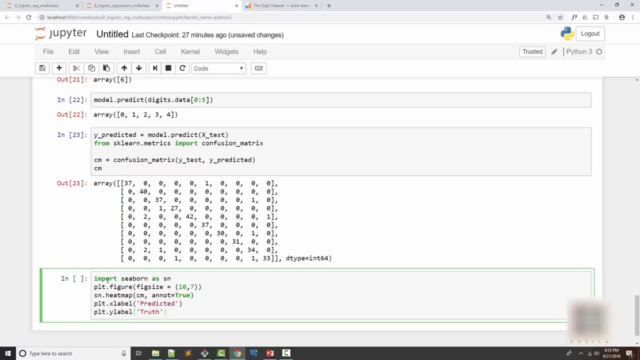 lib or seaborn, right, so i will use that library for the visualization here. i'm just going to copy paste the code for confusion matrix visualization. here i'm using seaborn library, which is similar to matplotlib. it's used for visualization and i'm calling a heat map here. 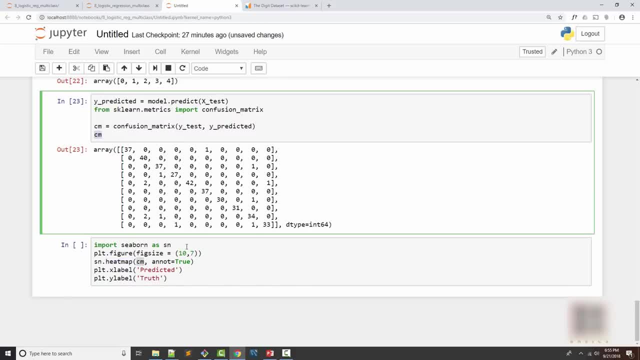 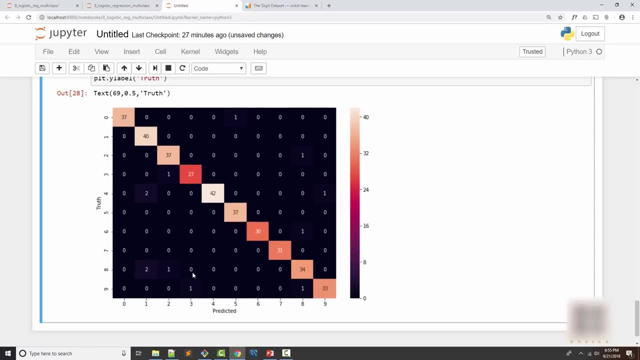 with the confusion matrix, cm variable that we created here, and when you run that, this is the confusion matrix that you got. now the way this works is see here. you see 37 number. what it means is 37 times the truth was zero and my model predicted it to be zero. 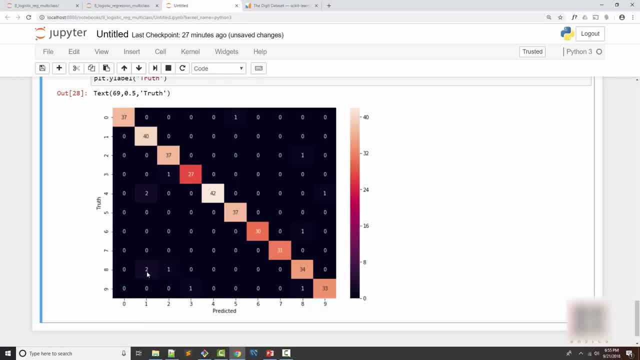 here. this two means two times. my truth was eight, meaning i fed my model the image of eight but pretending it was on the other side of the line. my model said no, it is one. so these are the instances where it's not doing good. so you can. 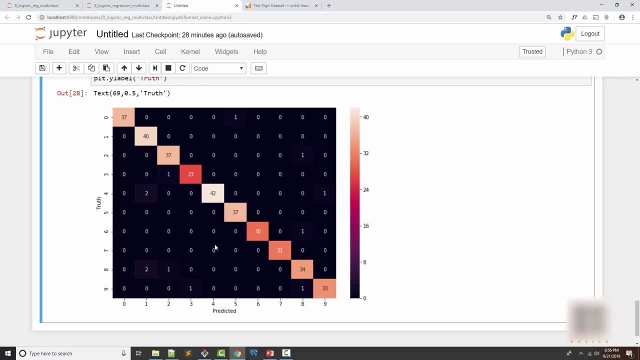 see that in, in anywhere in this area. in this area, when you don't see zero, it means your model is not working right. so here, for example, again two times, my images were of digit four, but my model predicted it to be one. so that's what this is. so confusion matrix is just a nice way of visualizing. uh, how. 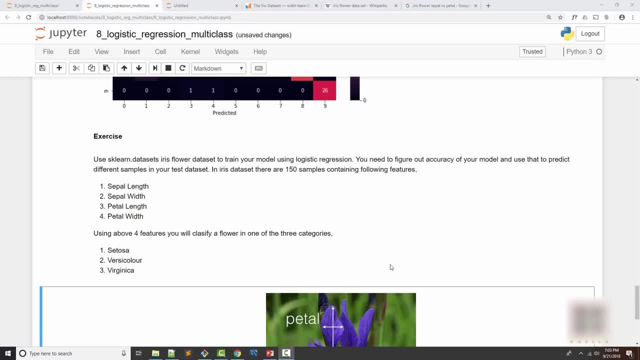 well, your model is doing all right. now it's the time for exercise. today's exercise is going to be using sklearn datasets, iris flower data set, which has following four features. so, if you don't know about iris, iris is a type of flower and the flower has a